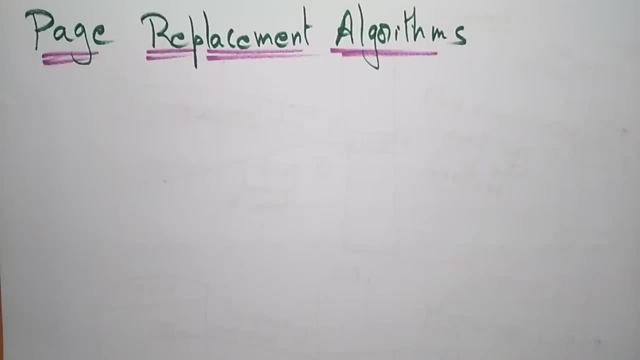 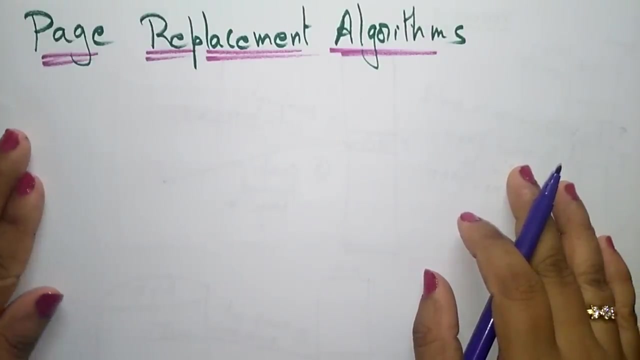 hi students, welcome back. coming to the next topic, that is, a page replacement algorithms. so the page replacement algorithms use it to. we have to which frame to has to be replaced and want, uh, which replacement algorithm shows the lowest page fault rates. so that will be decided with the help of this page replacement algorithms. so actually, this page replacement algorithm decides. 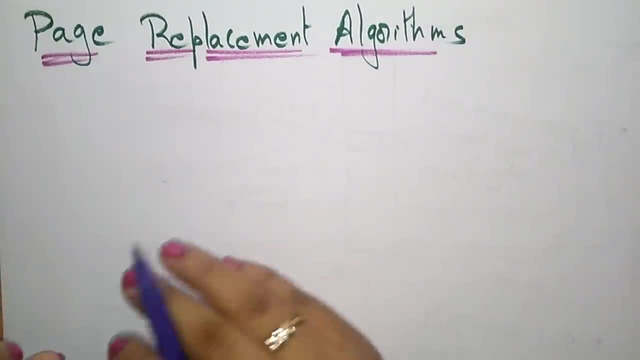 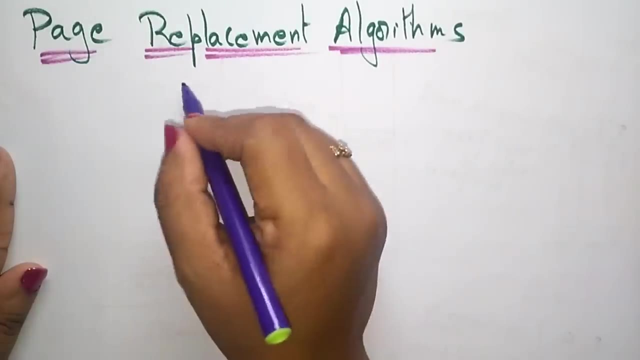 which memory, page to page, will be swapped out when a page of memory needs to be allocated. so there are three techniques that, uh, we use three different algorithms that we use in the page replacement algorithm. one is fifo- first in, first out algorithm, and then least recently used. 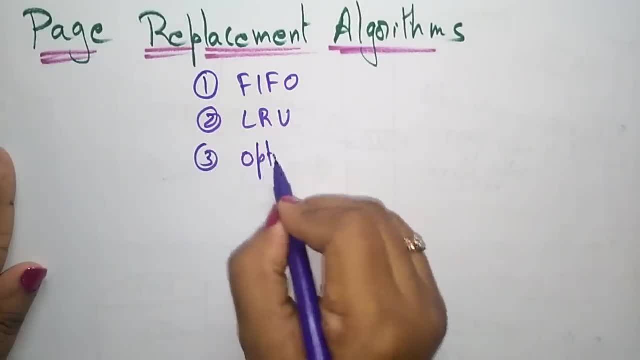 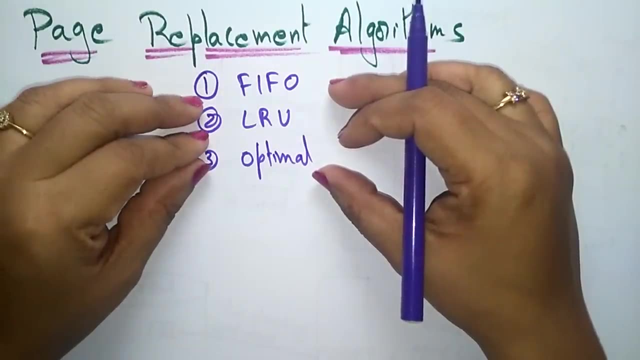 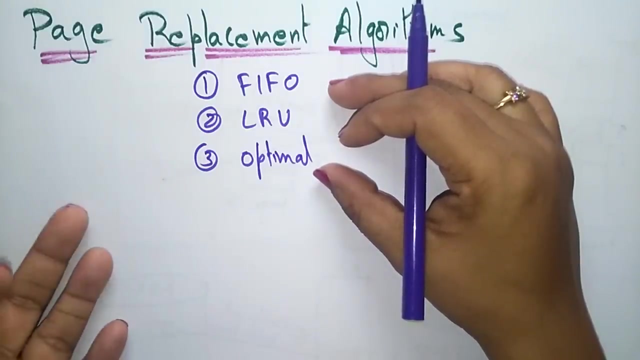 algorithm lru and the optimal. so these are the three uh replace page replacements algorithms. why we are using this? uh, three different algorithms? because, uh, with the help of these three different algorithms, we can find out which replacement algorithms occurs the uh less page faults less, uh, less errors like that. okay. so hit ratios and 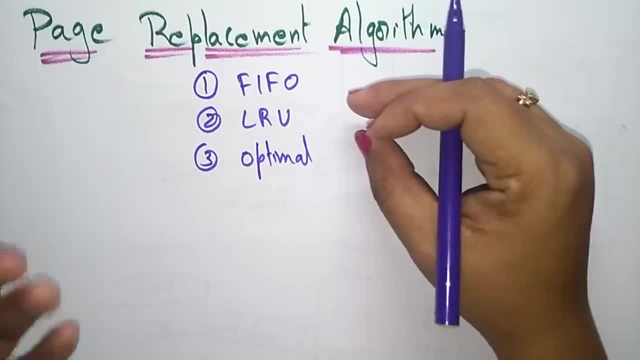 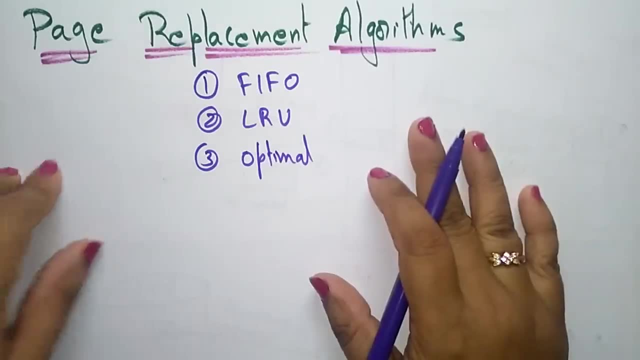 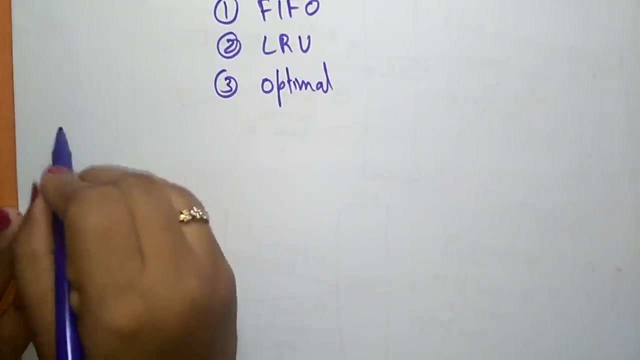 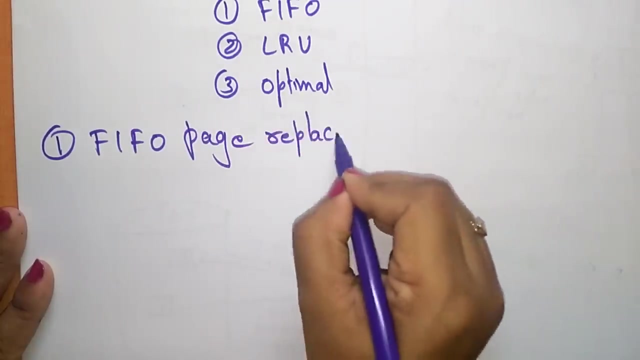 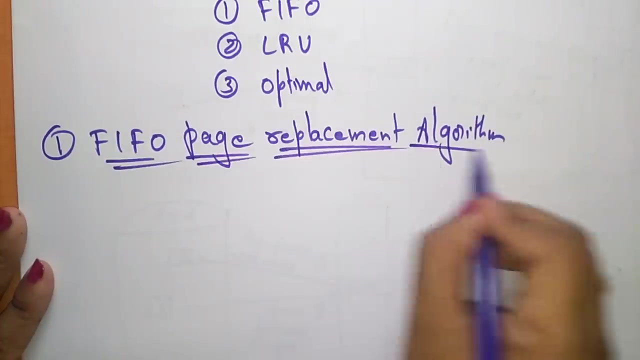 the miss ratios can be calculated. based on that values we can select the best algorithm. so the paste. these are the three different page replacement algorithms. now let us see the first page replacement algorithm. that is the first in first out, first in, first out page replacement algorithm. so the name itself is in saying that it is the first in first out. so whatever the first, 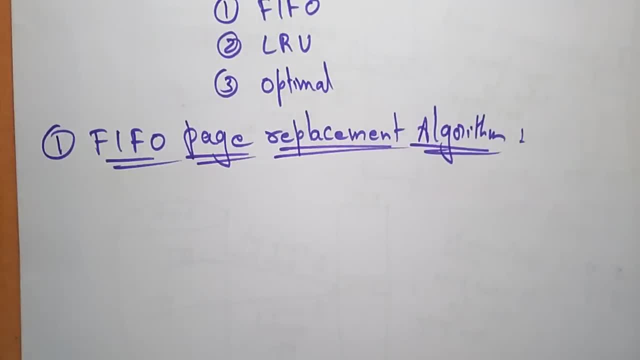 we are enter, enter into this the page. that page has to be deleted first. so it is very, is it very, easy to implement. before page replacement algorithm selects the pages for replacement that has been in memory for longest time. so replace the pages, replace the pages that has been. 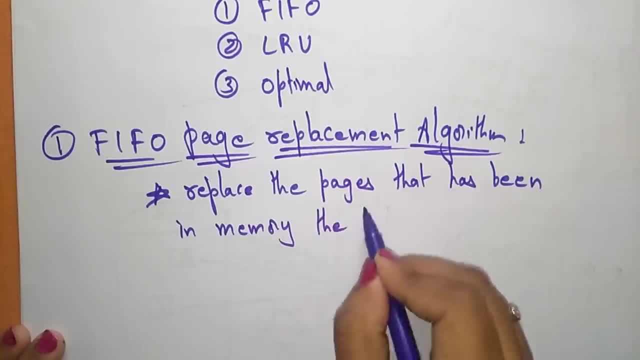 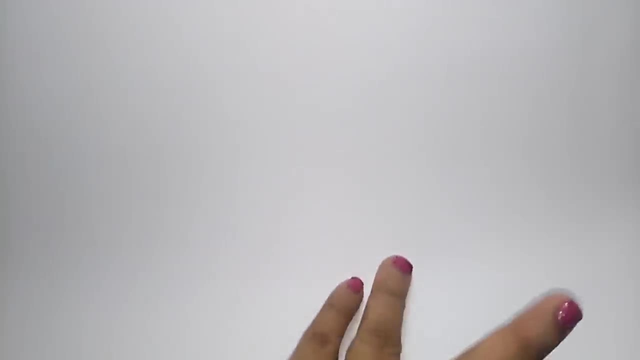 in memory the longest time, so the longest time goes to the page or the page that is in the memory for the longest time be loaded. the page recently bought. it is removed. let me explain with simple example. let us consider an example, how this- the first in first out page replacement algorithm will work. so let me explain. 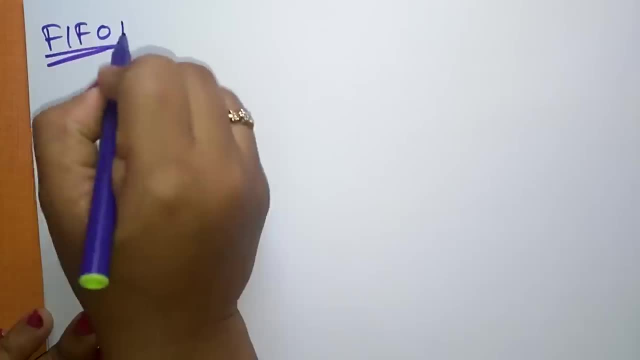 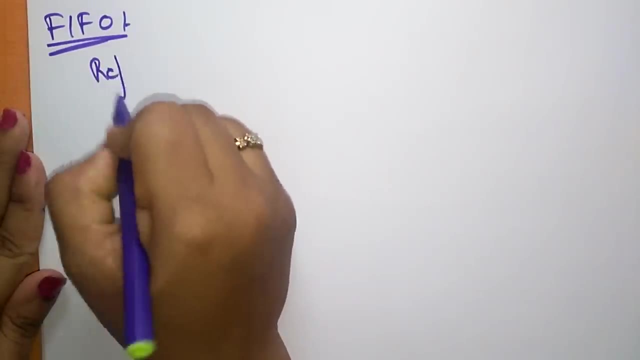 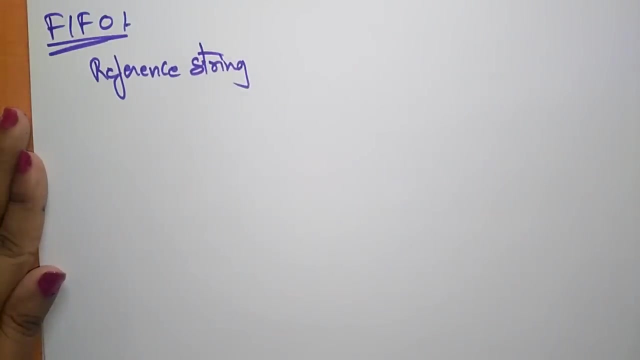 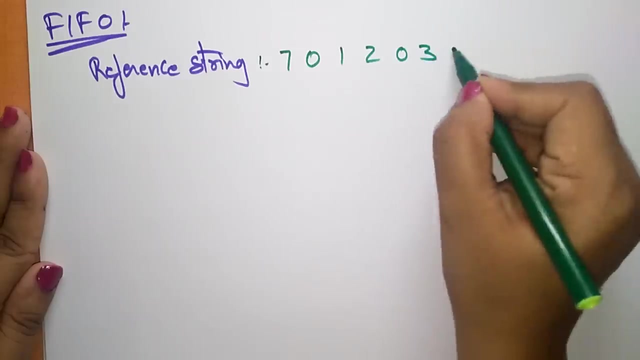 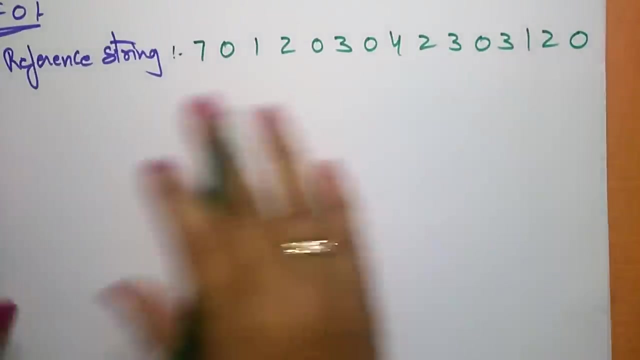 the FIFO example. now let me I'm taking some reference string. so reference string I'm taking here is seven zero one two zero three zero four two three zero three one two, two zero. so these are the pages that were present in the process. let us take this is a string. these 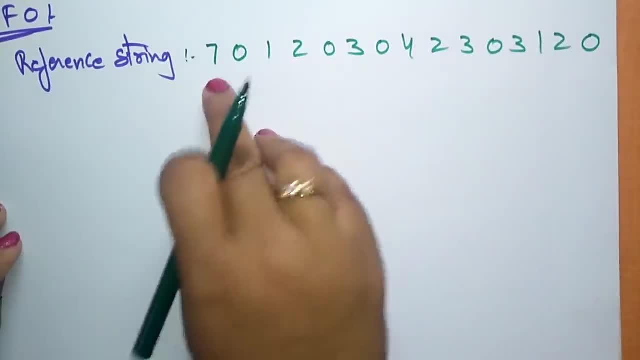 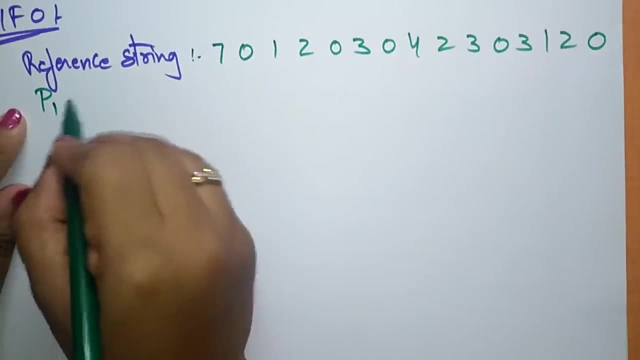 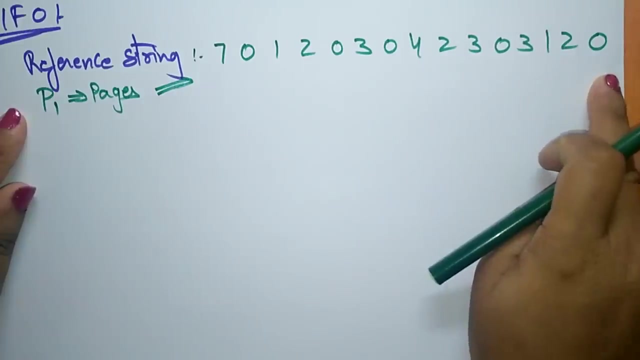 are the page numbers, Pages that the CPU is demanding. the CPU is demanding further this Pages. let us take the p1 process. so this p1 process consisting of pages, so these are the pages that are present in the means main memory. so the main memory data time can't store. 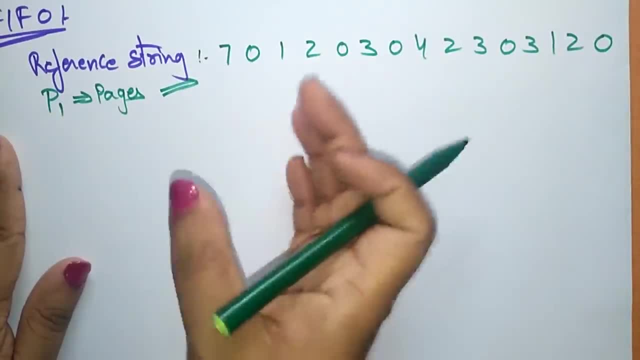 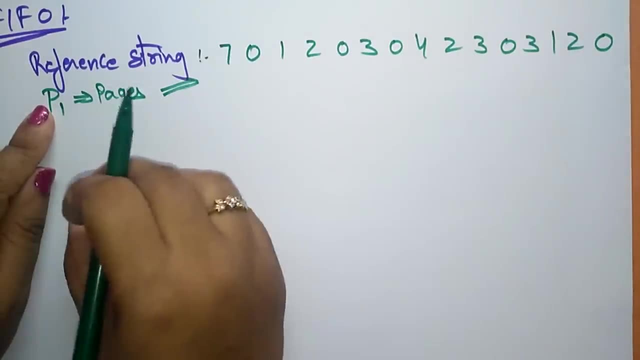 all these pages. so let me see p1 process mask at first. so let me progress this. and now it's Because the main memory size is less when compared to the logical memory. Now the CPU is demanding the page numbers, So based on the page. whenever the CPU is demanding the page, it has to check that page is present in the main memory or not. 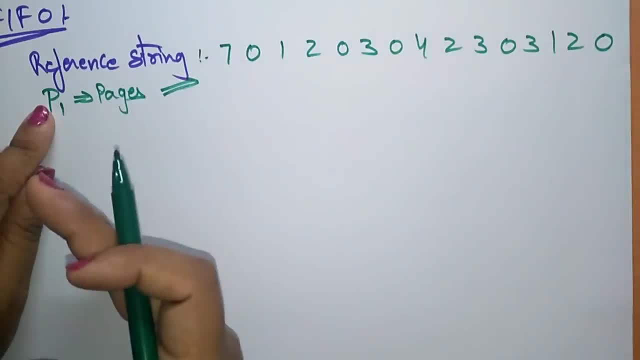 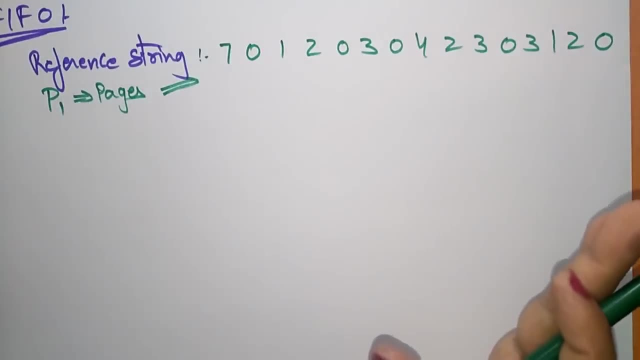 If it is not present in the main memory, it has to get from the secondary memory and store it in the main memory. So that is a page replacement concept. So here, while it is, if the page is not found in main memory, then we call it as a page fault. So that we already know Whatever the CPU is demanding for the page. if that page is not present in the main memory that you call it as a page fault. So whenever the page fault is occur we have to bring that reference page. 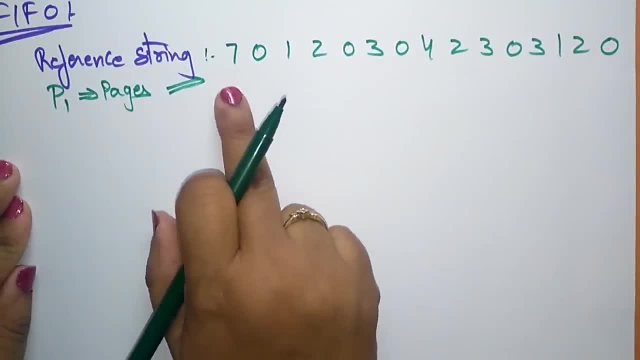 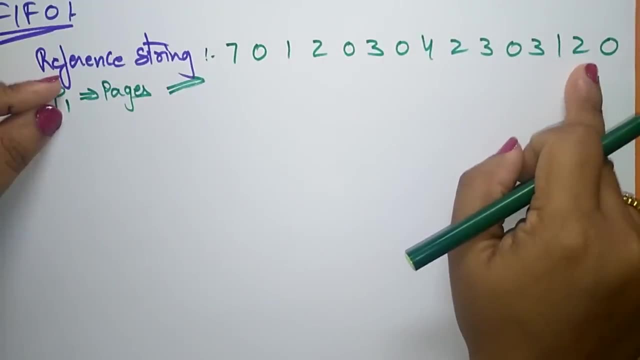 So these are all the reference pages the CPU is demanding. So these reference pages are nothing but the process. P1 holds these reference pages. So this is the reference pages. So this is the reference pages. So it has to bring that reference page which is demanded by the CPU from disk. 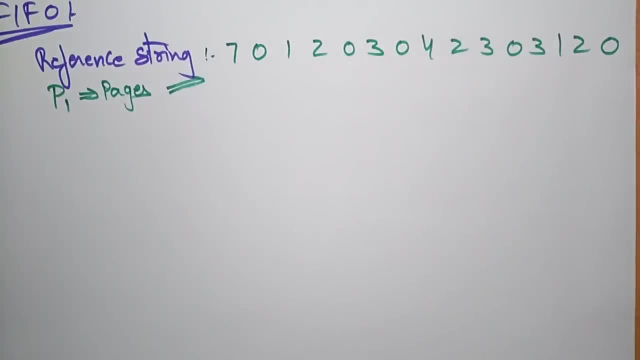 So every time getting that from the disk is when compared to this is if the page faults are more than the CPU time is wasting. So because the disk is slow when compared to the main memory. So every time if the page fault is occur you call it as a page fault. 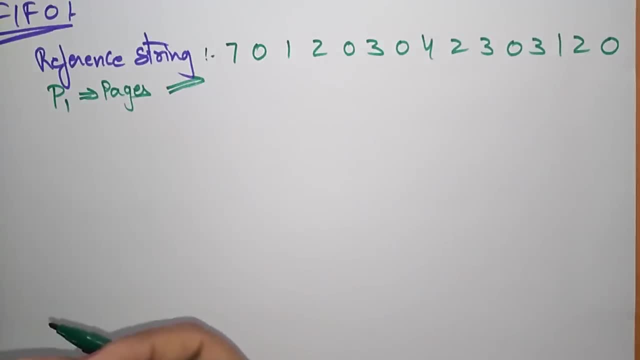 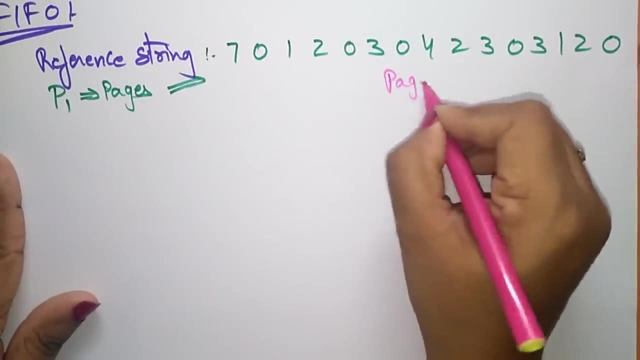 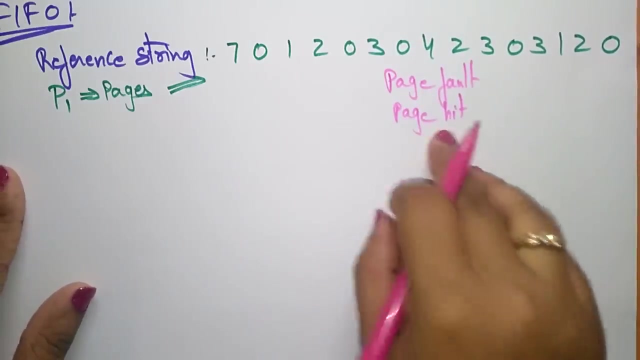 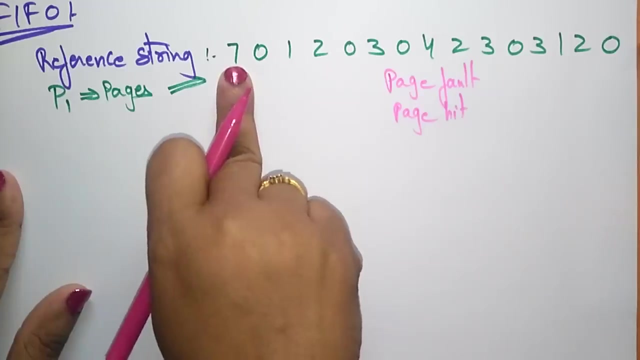 If there is already the page is present, if that you call it as a. So sometimes you came across in this while you're discussing about this algorithm- that is a page fault And page hit. So page hit means whatever the page that is demanding by the CPU. if that page is present in the main memory, that you call it as a page hit. 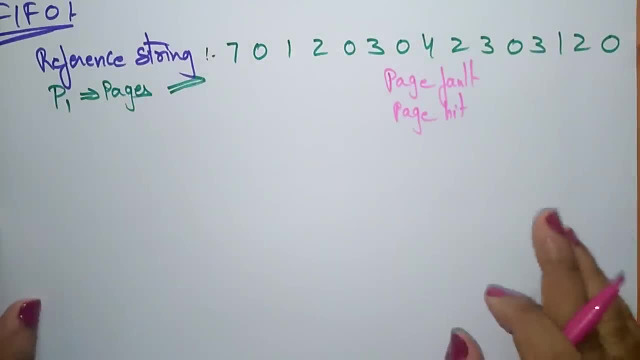 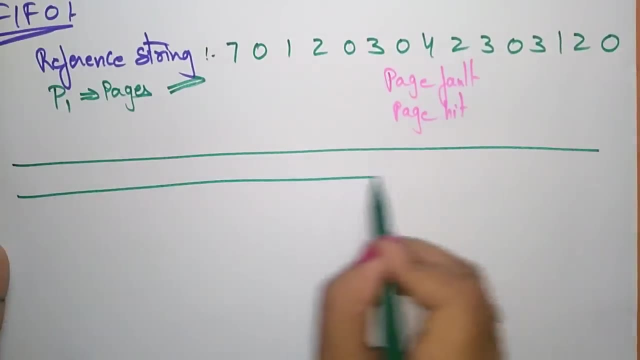 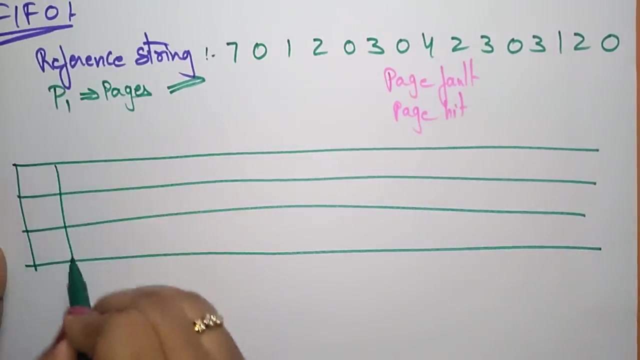 If the page is not present in the main memory that you call it as a page fault. So let me explain that. So let us take. So let us take: the main memory is having holding only three frames at a time, Only three pages at a time. 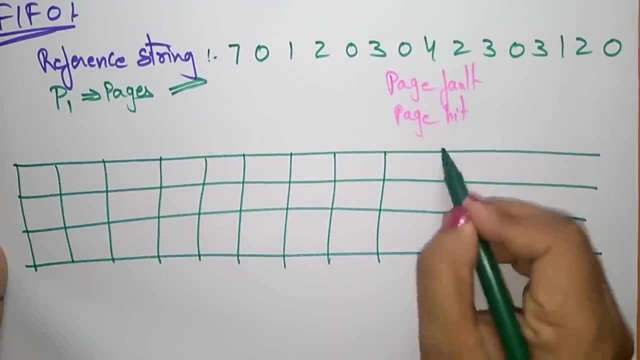 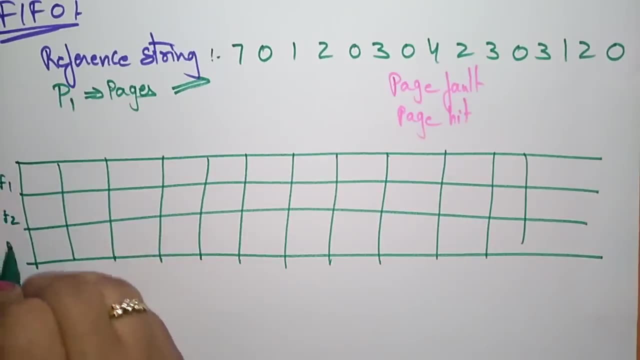 Not a day. So that is only the main memory capacity I'm talking about. So this is a main memory. here It's having the frames frame one, frame two and the frame three. So don't be confused, See clear. So this is a frame. 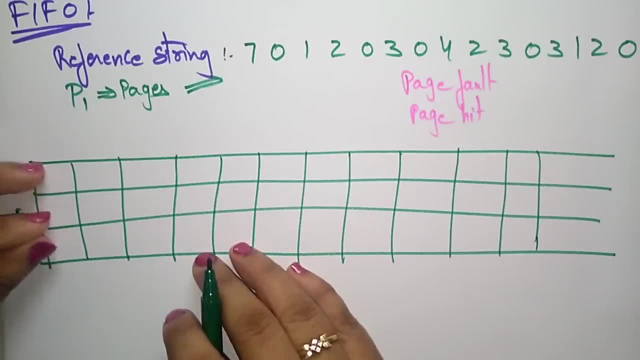 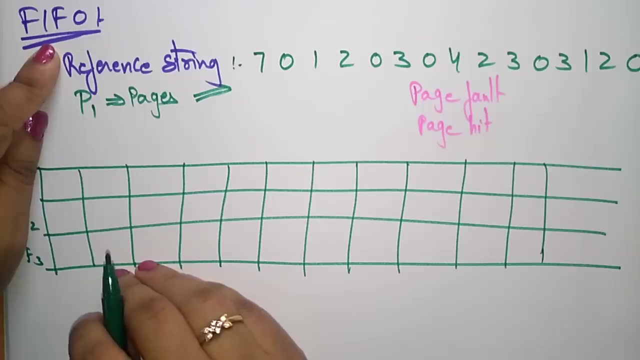 This is a main memory, So the main memory can hold only the three pages. Only it can hold three pages. OK, So if if you want to store another page, it has to be replaced How it is replaced, by following the concept first in, first out. 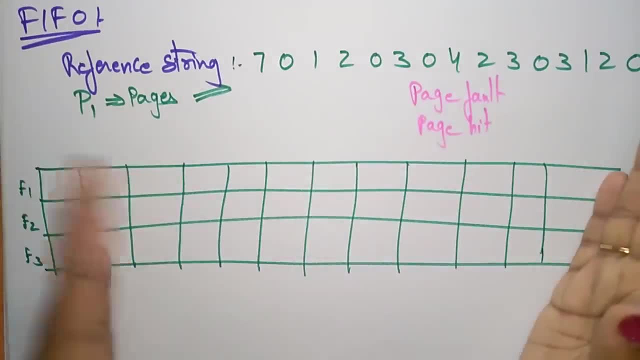 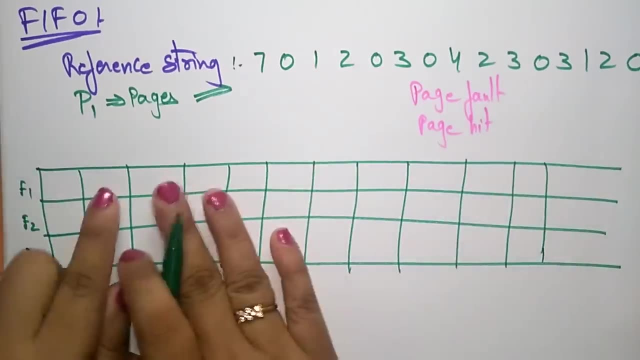 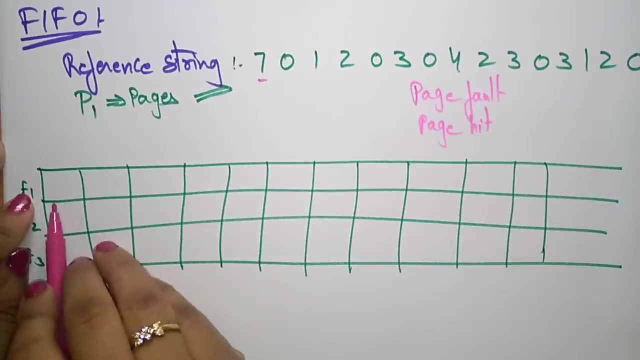 OK, So starting the main memory is always free. So whenever you are starting the system or the main memory- that is, a RAM- is free. So means now the CPU is demanding for First, it demanding for seventh page. so it checks in the main memory. the CPU is demanding. 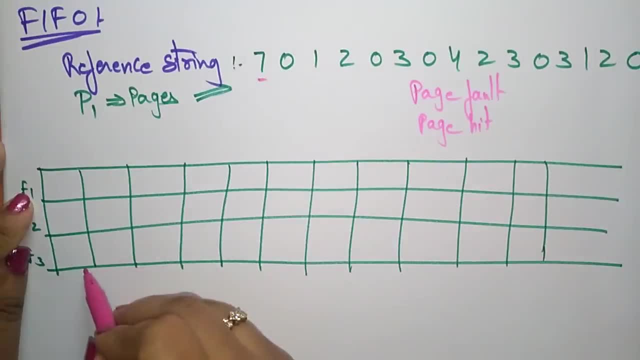 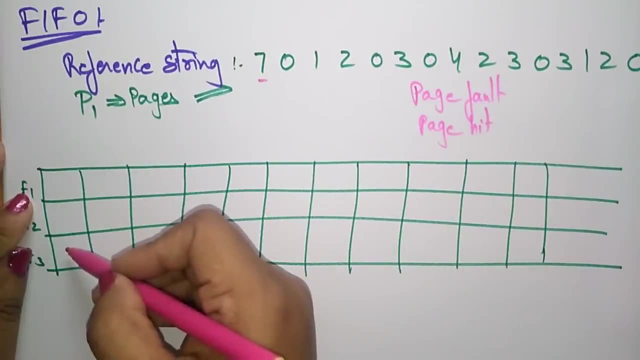 the reference string, that is a page seven, that it is not present in the main memory. OK, The first. it is free. So seven is not here. So whenever the seven is not here, what the CPU will do? the control transfers to the operating. 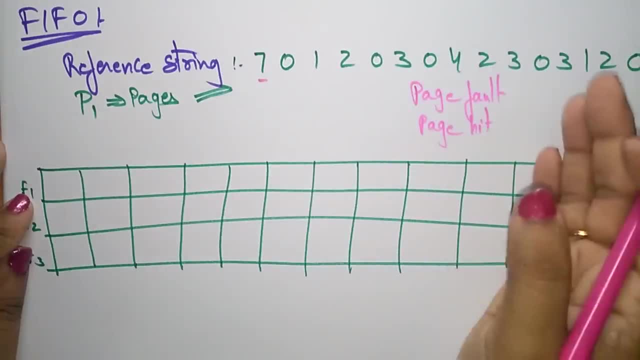 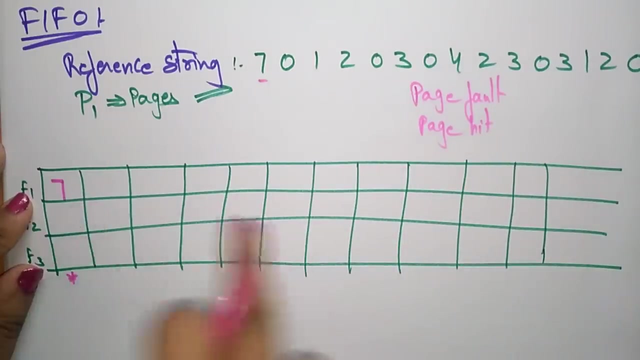 system and from operating system to the disk, the disk. from this we are getting the seventh page and place it in the main memory. So this is page fault, because seven is not there in the main memory. So this is the main memory here seven is not there, we are getting from the disk. 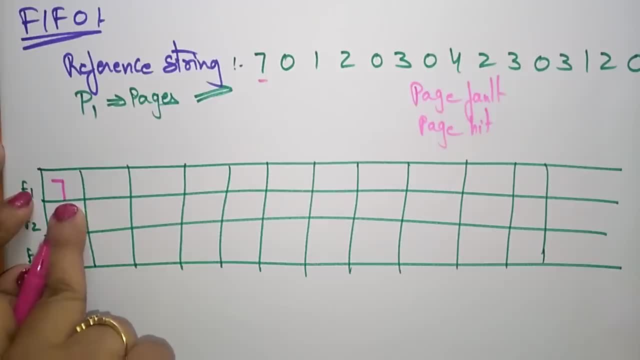 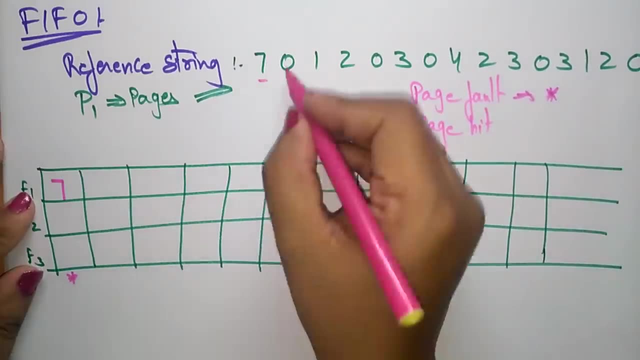 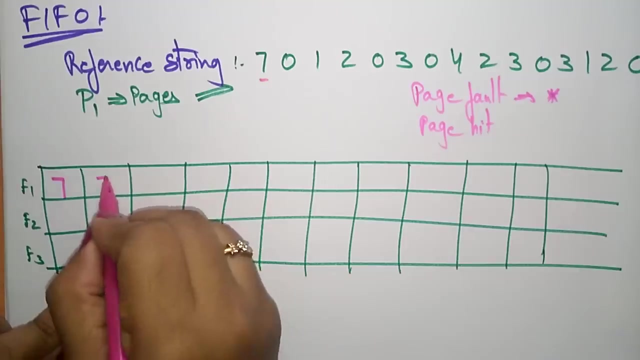 So if the page is not present in the main memory, that you call it as a page fault. So the page fault is indicated with Start. next, the CPU is demanding for the reference string. next, zero. OK, zero is not present in the main memory, So this is also. 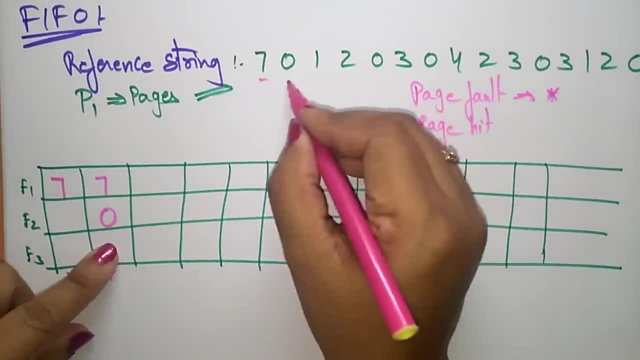 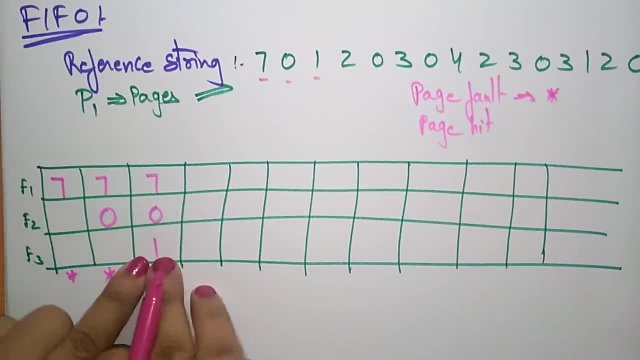 OK, Page fault, So next one. So one is also not present in the main memory, So we are getting from the disk. OK, So now I want to store the two. So the CPU is demanding for the two in the main memory, but it is not there in the main. 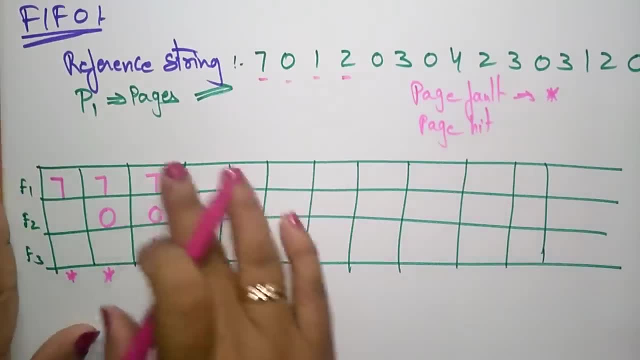 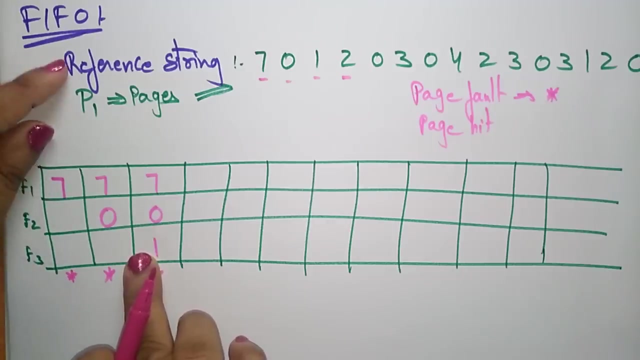 memory. So obviously it is page fault only, but already the main memory is full. The main memory, Whatever, it is Full. So what it will do? so it has to replace the page which is not using. So the what this concept before will do, first in, first out. 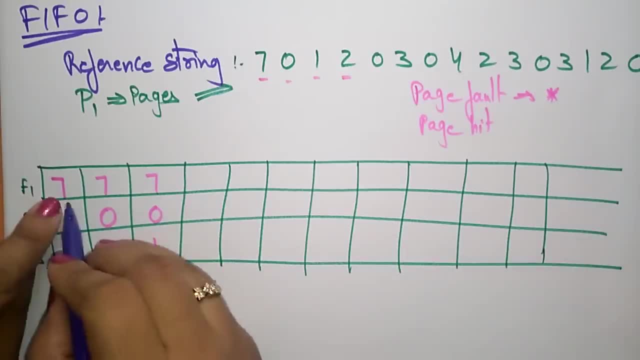 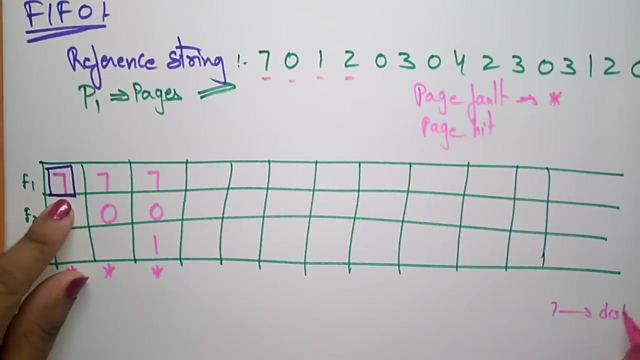 So what is the item that is placed in the first? The first item that we placed in the memory is seven. So the seven has to be replaced. So the seven has to be replaced. That is Swap. The seven is Swap. 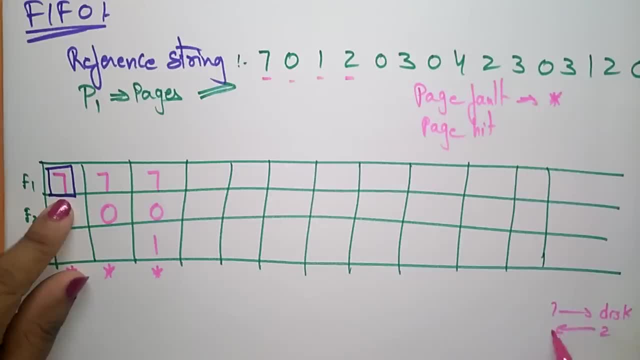 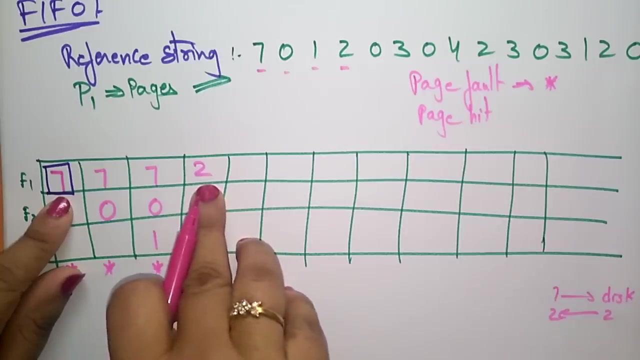 And from disk. The two will be placed in the place of seven, So it is just swapped to the disk and then from this we are getting the two, Two Zero One. So this is also page fault, because two is not present in the main memory. 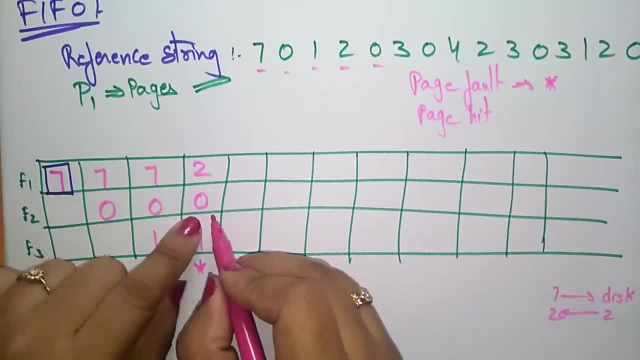 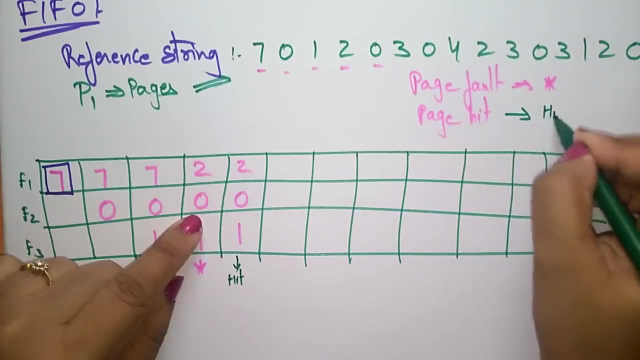 So after two I have to place the zero, But the demanded page, that is already present in the main memory, So no need to bother about So this you call it as a hit. If the demanded page is present in the main memory, that you call it as hit. 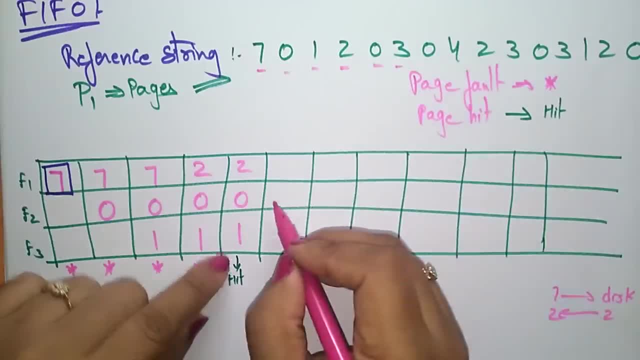 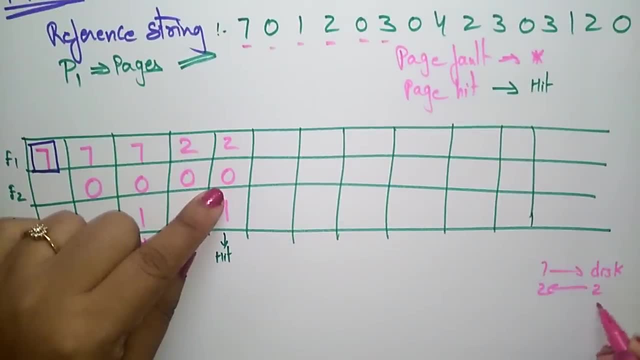 So next Three, So the three. the CPU is demanding for the three, So the three is not present, So we have to get from the disk. So which page I have to be replaced? The next, The first in first out. The seven is: 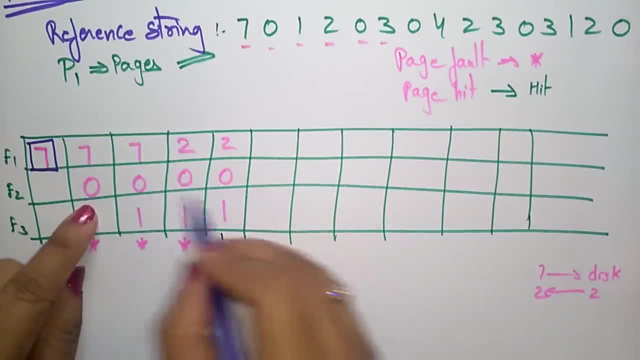 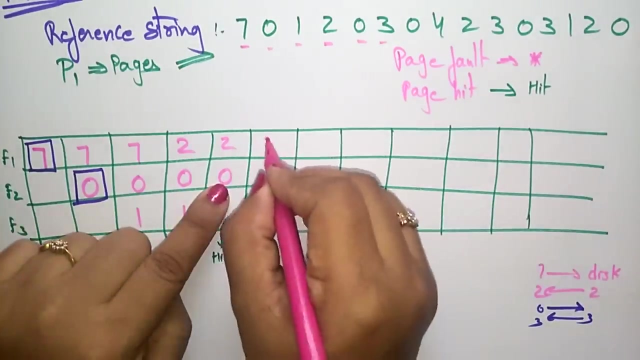 is first in, first out. So this is already remote. So next is 0. So the 0 has to be sent to disk and from disk we are getting the 3 value. Okay, So in place of 0 I have to place. 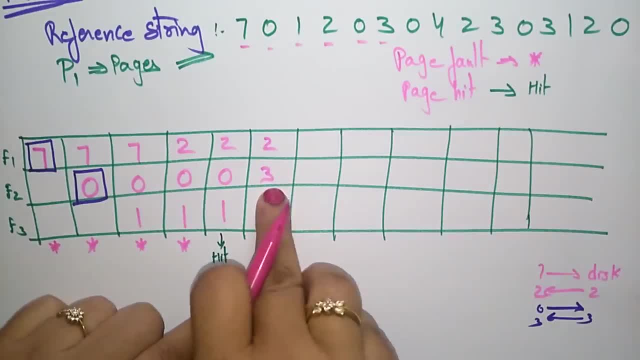 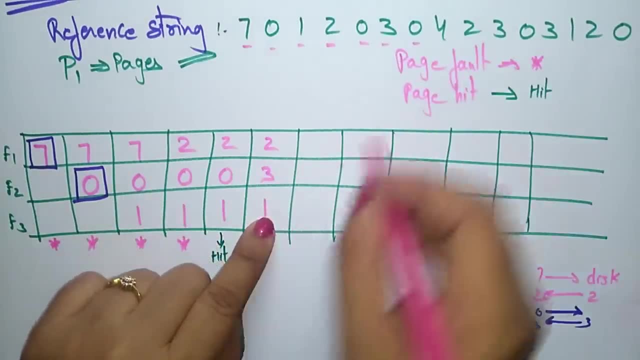 3, 1.. So this is also page fault, because 3 is not present in the main memory. So next I have to place 0.. So in which place I have to place 0?? I have to replace 1.. So the next. 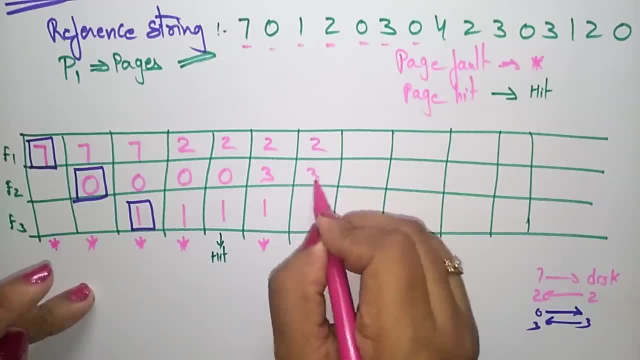 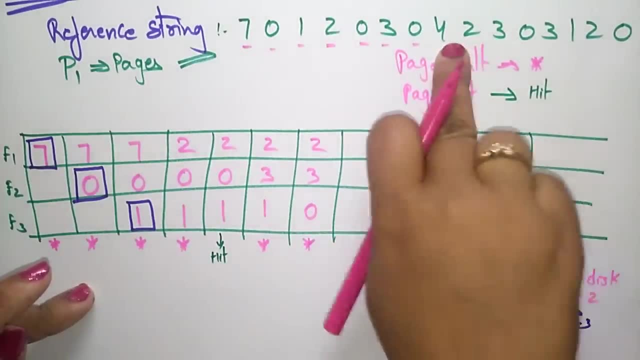 first in, first out is 1,, 2,, 3, 0. So this is also page fault, because 0 is not present in main memory. So next I want to place 4.. Okay, So, which I have to be replaced, So I. 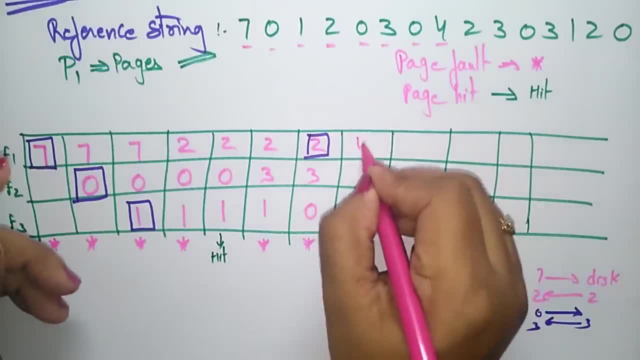 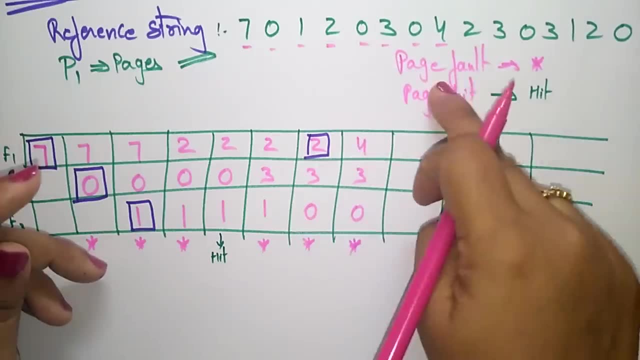 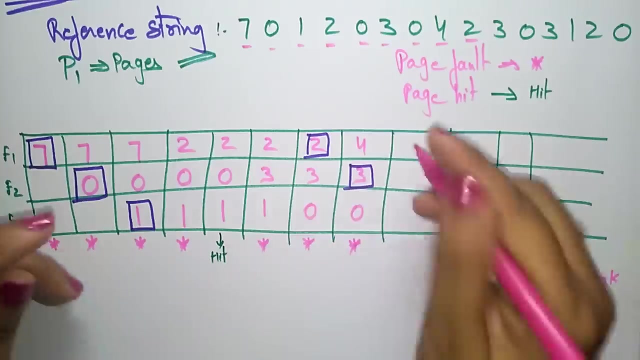 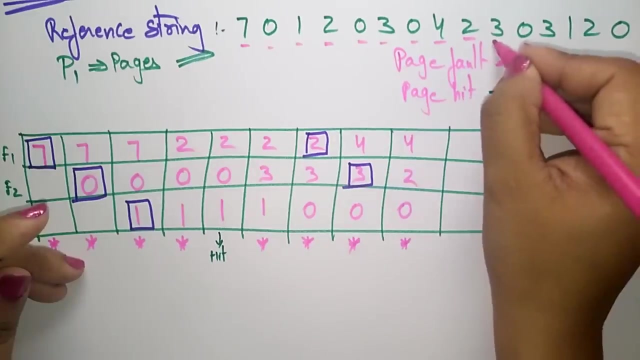 have to replace 2.. So 4.. 4, 2, 0. So this is also page fault, because 4 is not present. Next, I have to place 2.. Now 3 has to be replaced 4, 2, 0. So this is also page fault. Next, 3. This page has. 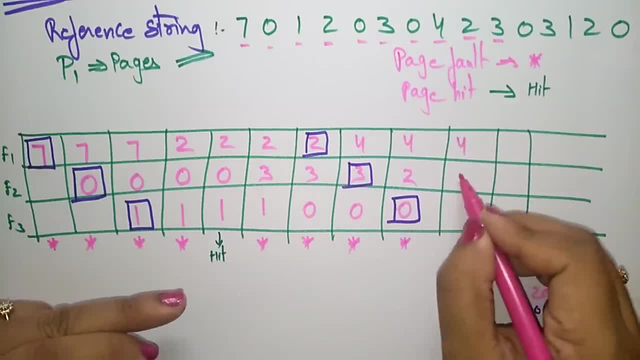 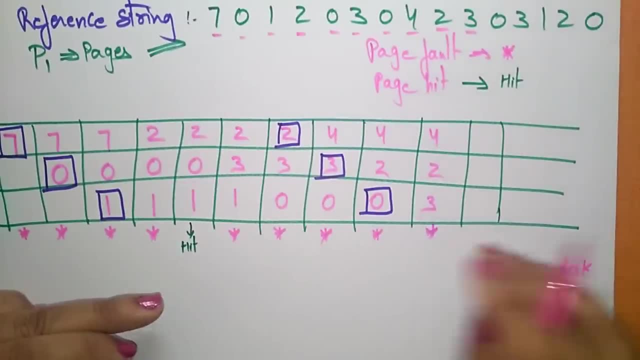 to be replaced 4, 2, 0.. Okay, So this is also page fault. Next 3.. This page has to be replaced 4, 2, 0.. So 3, 2, 0.. So this Is also page fault. Next 3.. This is also page fault. Next 0.. So the 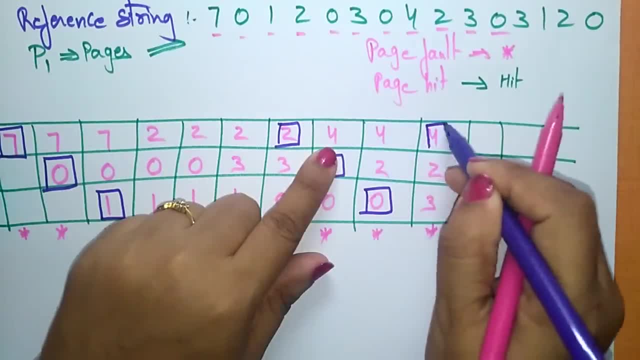 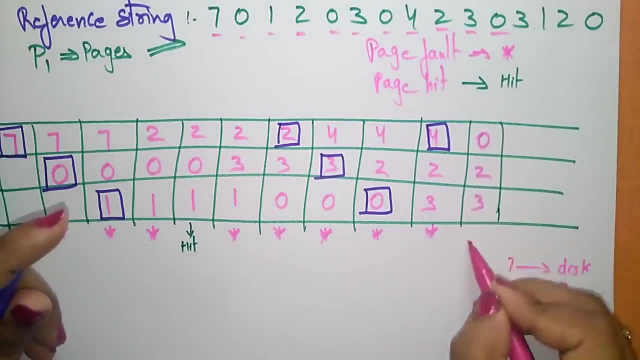 first in, first out. what is this? 4 is first in, so that has to be replaced. Now place 0,, 2 and 3.. This is also page fault, because 0 is not present. Next, I want to place 3.. 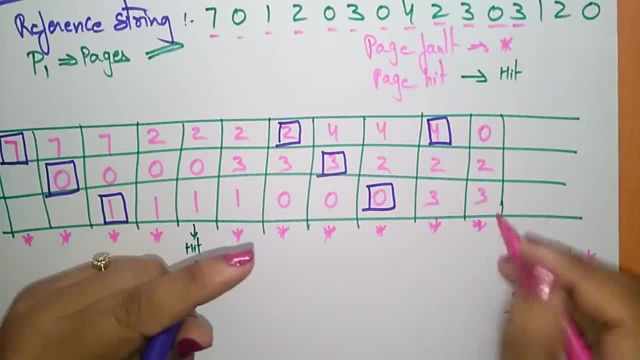 But 3 is already present in the the demanded page by the CPU as code base. So again, 1 is not there. Now I have to place 1.. So that shall be replaced. Now I have to place 2.. Next, where is 0.. I have to place 0.. I have to replace 3.. Next, I want to place 1.. I am. 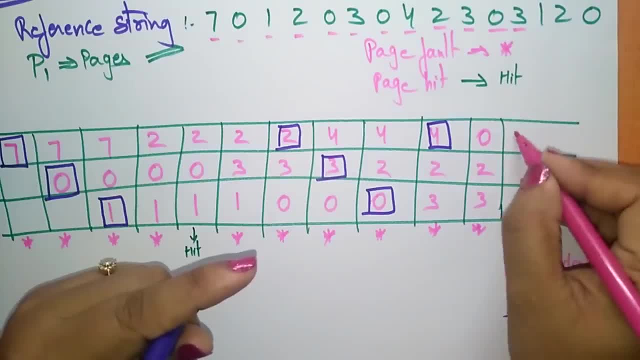 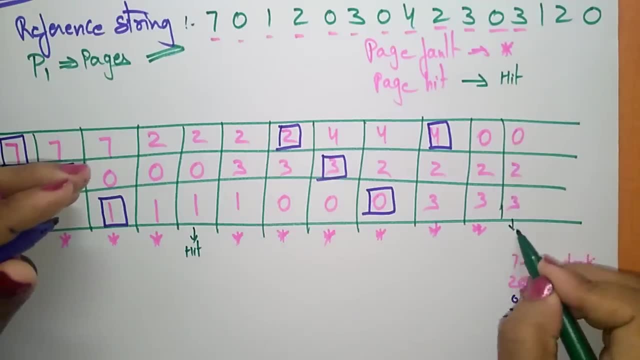 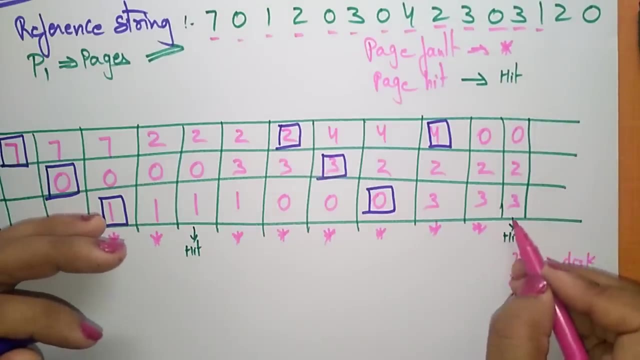 CPU3, that is, 3.. The 3 is already present in the main memory, So just write 0,, 2,, 3.. So this you call it as hit. So next, 1.. Which place I have to be replaced? The 2 has to be replaced because 2 is staying in long time. 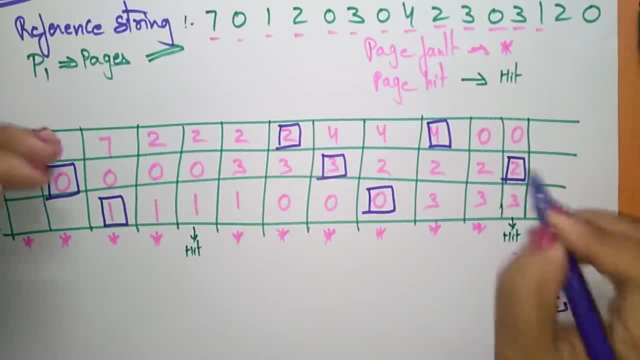 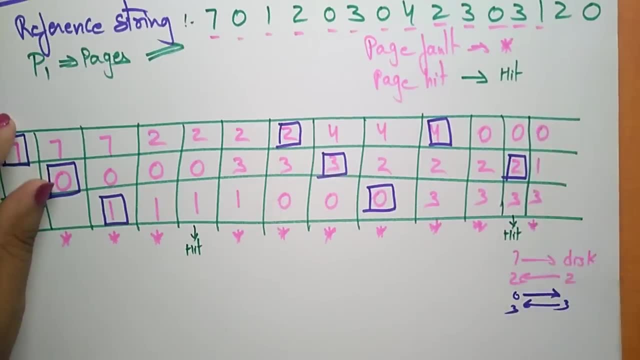 So the 1st in page is 2.. 2 has to be replaced, So 0, 1, 3.. This is also page fault, So next I have to place 2.. Which place has to be replaced? So 0, 1, 3.. So the 3 is staying in long time, So just replace 3.. That is 0, 1, 2.. 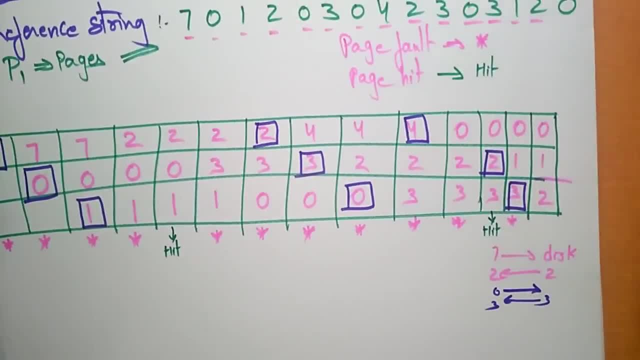 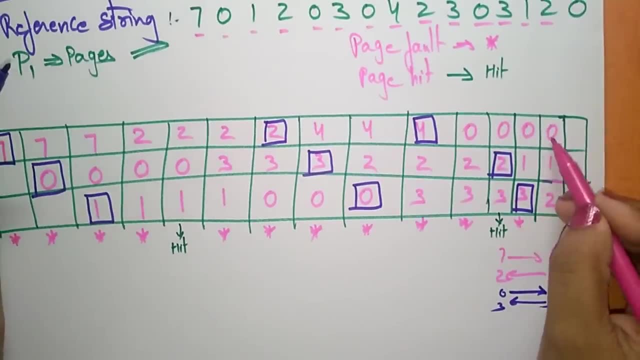 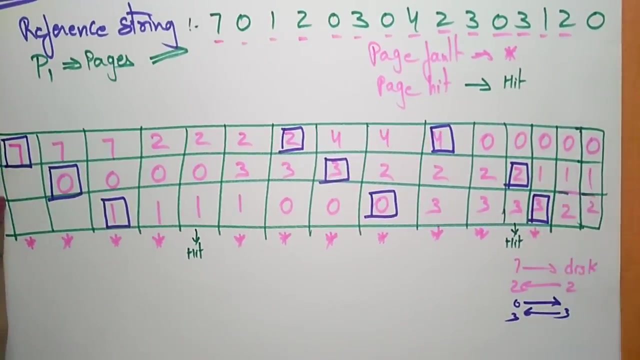 Ok, Ok, Ok, Ok, The last page. What is the last page? The last page that is demanding the CPU is 0. But 0 is already present in the. the demanded page is already present in the main memory. So just write So this. you call it as hit And this is page fault. So the star marks is called as a page fault and these are the hits. So we can, by seeing this, we can observe that. 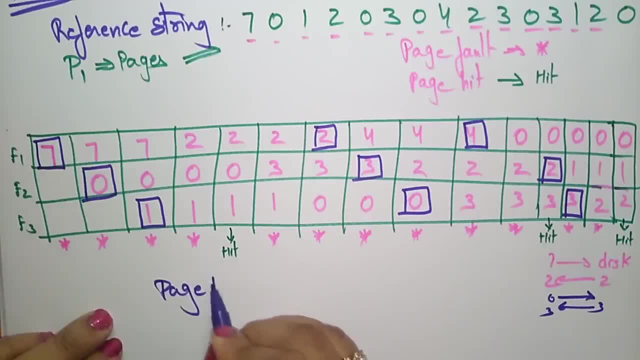 So this you call it as a page fault. So this you call it as a page fault, and these are the hits. So we can, by seeing this, we can understand that The number of page hits areêtes How many page hits are there? 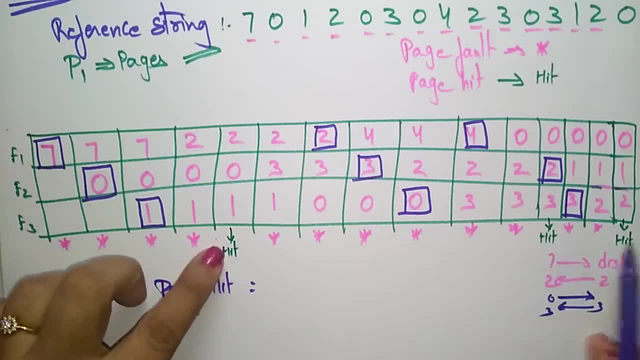 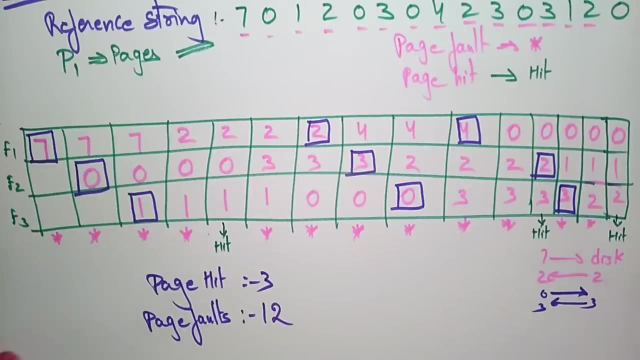 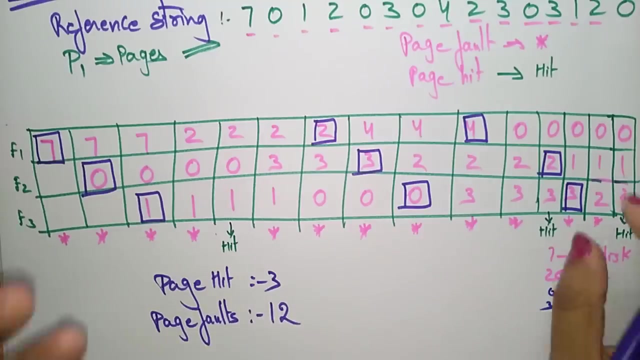 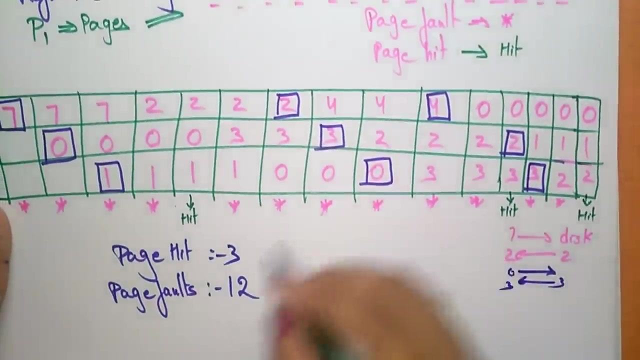 The total page hits are 3.. The total page hits are 3.. How many page faults are there? Problem, Problem, Problem, Problem, which all these FIFO algorithm is suits or not for our program. So actually the page faults can be calculated as, suppose, a hit ratio. 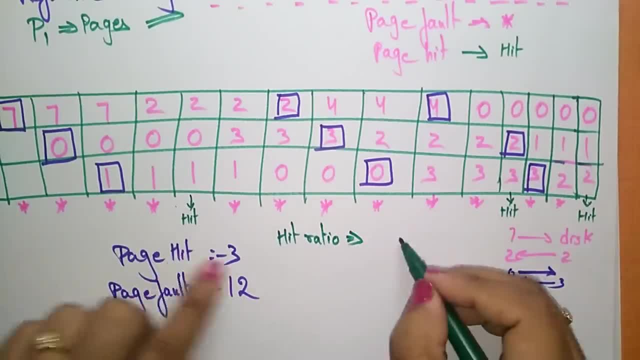 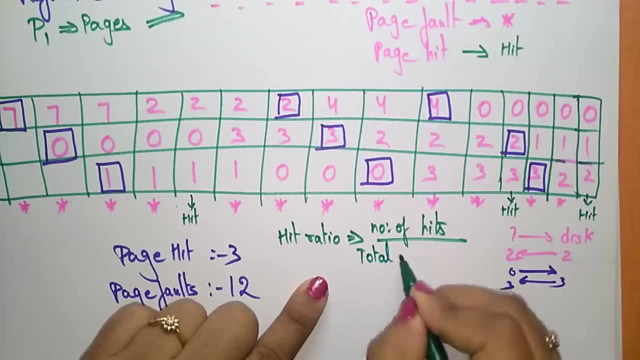 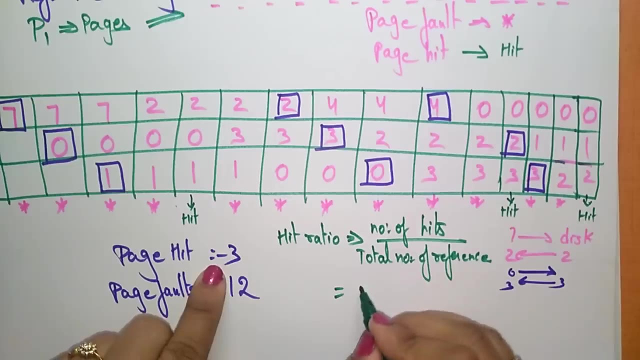 If you want to calculate the hit ratio. hit ratio can be calculated by number of hits, by total number of references. So this is a formula to calculate the hit ratio. So what is the number of hits? Number of hits are 3.. 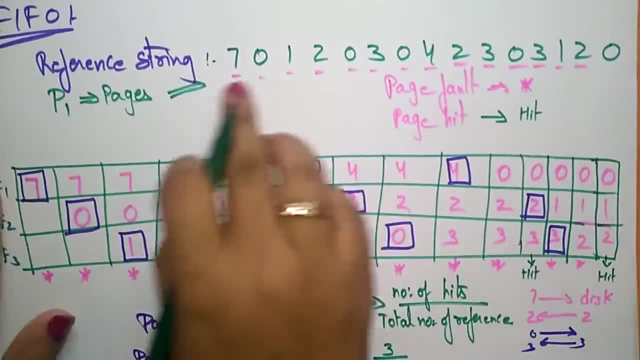 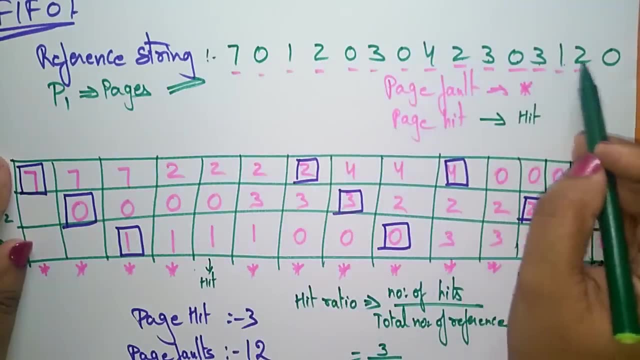 What are the total number of references, Means the pages that we are requesting? the CPU is requesting 1, 2, 3, 4, 5, 6, 7,, 8,, 9,, 10,, 11,, 12,, 13,, 14, 15..